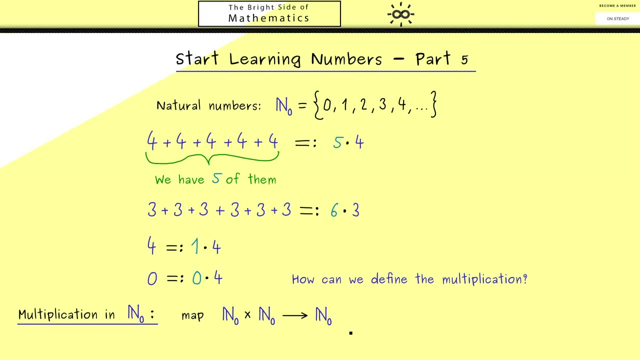 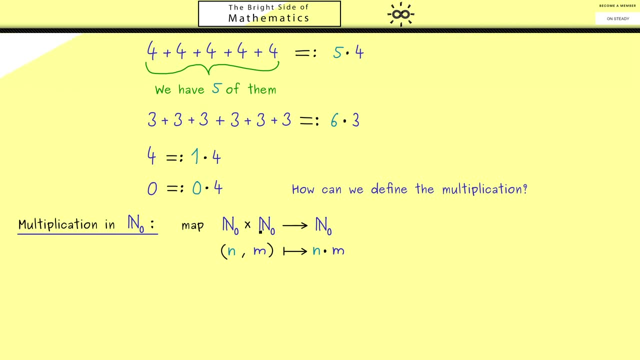 numbers as the input and one natural number as the output. Ok, and then in the next step we have to give the definition of this map. So maybe this looks all familiar because we had the same discussion when we introduced the addition, And indeed we can use a lot of things we've already learned In. 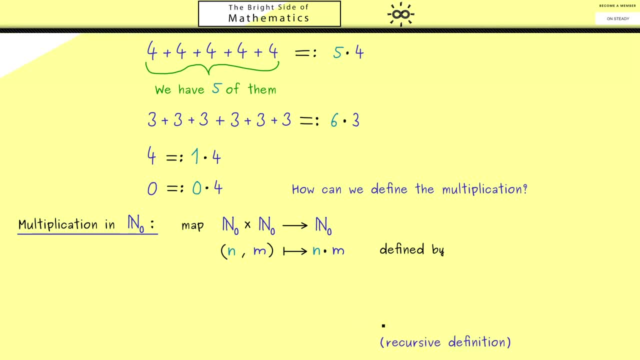 particular, we know we don't have to give an explicit definition. we can give a recursive definition. Therefore, we first have to say how the starting point 0 acts, And that's what we've already discussed. we should get out 0, no matter what m is. 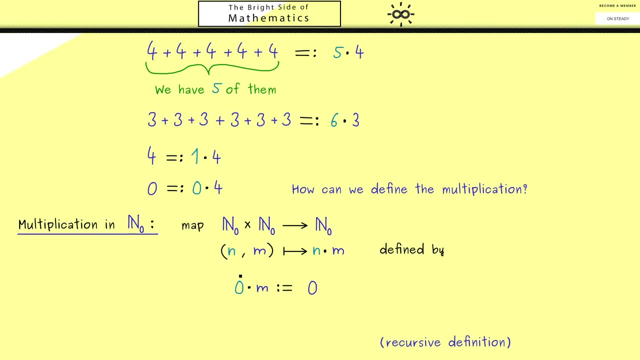 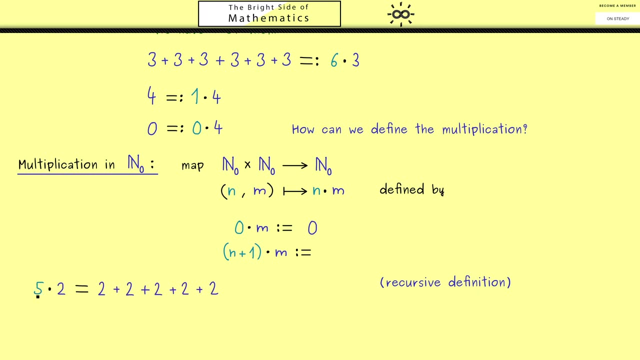 Now the second ingredient we need would be something that tells us how the successor of n acts. In other words, are we able to define n plus 1 times m? In order to do that, let's look at an example to see what we actually want. Of course, 5 times. 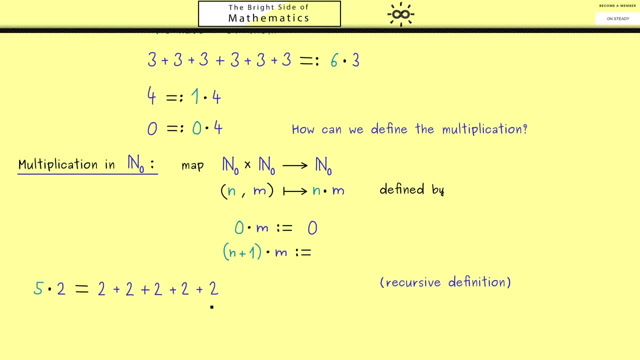 2 should be just given by the sum of 5- 2s. However, when we now add another 2, we should get out 6 times 2.. Ok, not so surprising, but here you should see the successor of 5.. And on the other hand, here we still have 5 times 2.. And of course, this is the. 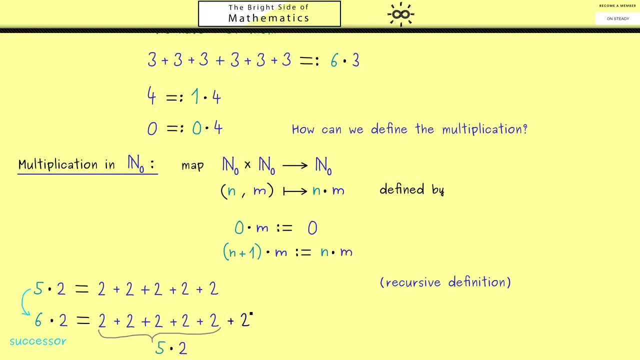 recursive connection we searched for. Therefore, in the general definition we would write: take n times m and add another m, And since we want to be completely precise, we set parentheses here. Certainly, you already know that we will just agree to say that the dot binds closer than the plus sign, and then: 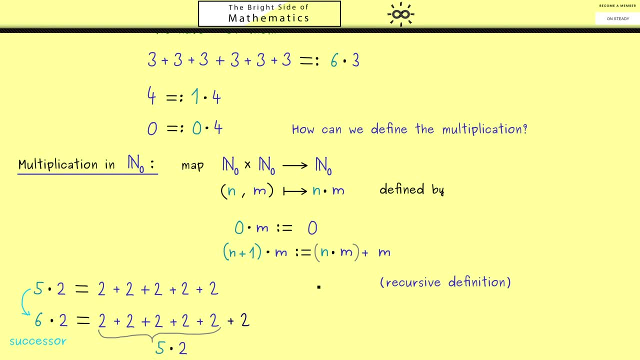 we can just omit the parentheses. This way, we can just omit the parentheses. This makes everything easier to read. Ok, summing up, here we have a recursive definition for the multiplication And by Dedekind's recursion theorem I showed you when we discussed the addition, the 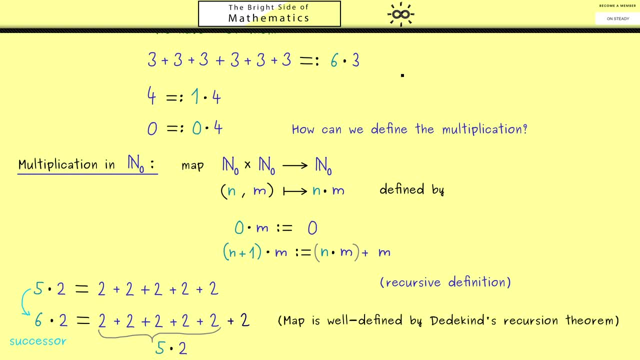 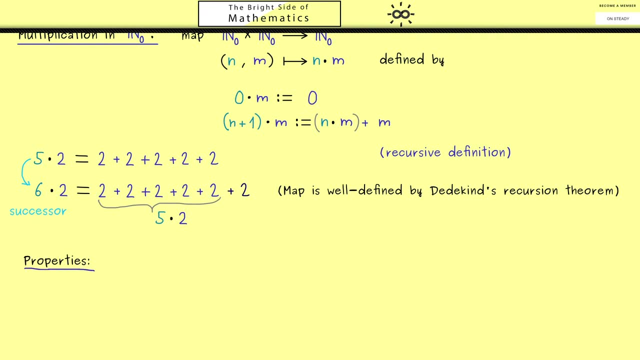 multiplication here is also well defined. Knowing this, let's discuss the properties the multiplication has to offer. Of course, they are similar to the ones we have for the addition. The first one is simply that for the multiplication of three numbers we can set the parentheses as a. 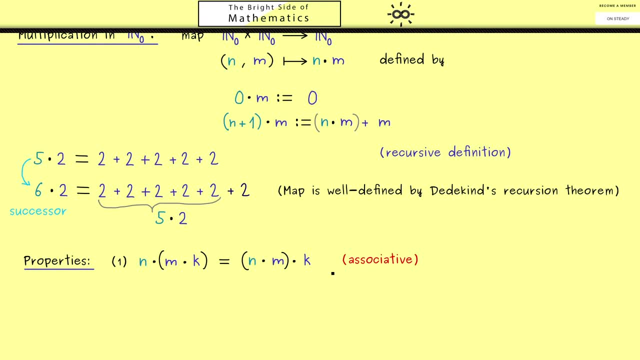 we want. As for the addition, this is known as the associative law, And the other law we got to know there was the commutative law. It simply tells us that we are allowed to change the order in the multiplication And the last one we 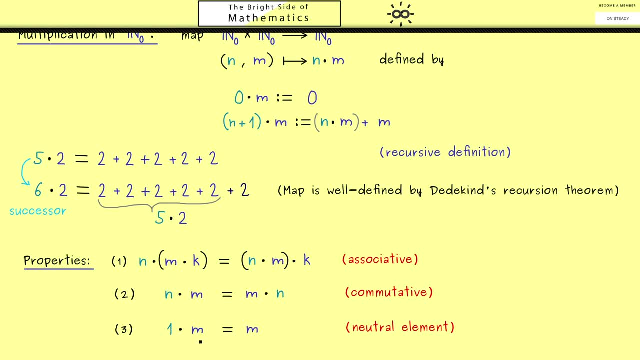 immediately get from. the definition is simply: 1 times m is always m, So we have the number 1 as the neutral element with respect to the multiplication. Now, please recall, with respect to the addition, this was the number 0. But otherwise we have the same calculation rules for both operations. 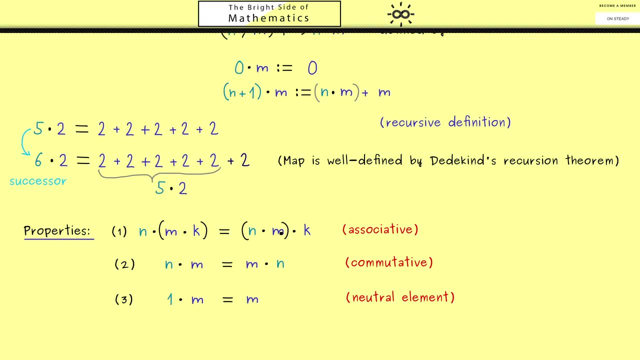 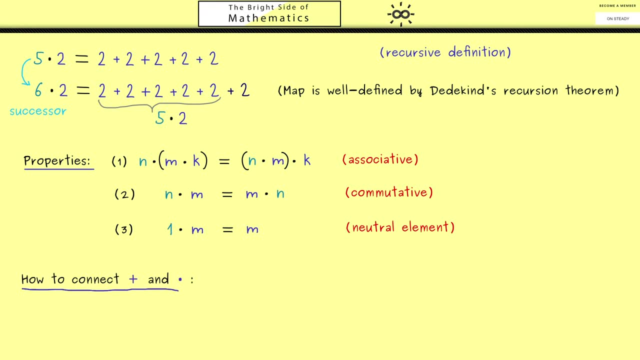 For this reason, a fitting question would be: how do we connect both operations? Of course, this is something you learn in school- how to deal with when you have addition and multiplication in one calculation, Or, in other words, how can we rewrite an expression like this- And of course, you know it, you can expand it. 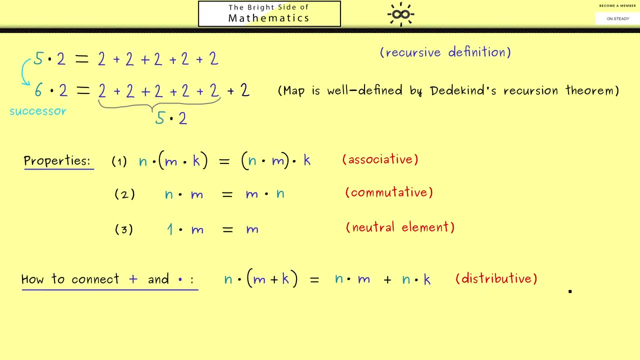 like this And we call it the distributive law For this. maybe it's a good idea to use the distributive law To write down the proof by induction. Now, the variable we do the induction for should be again n. Therefore the base case would be starting with: n is equal. 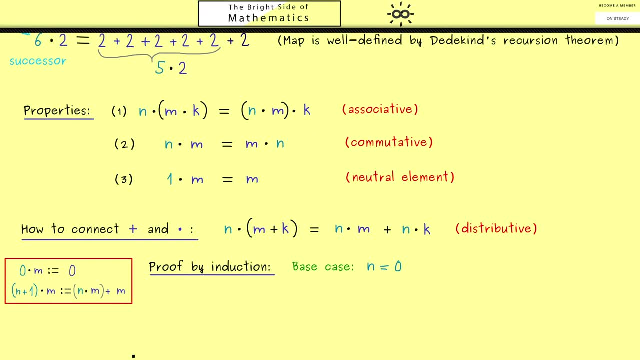 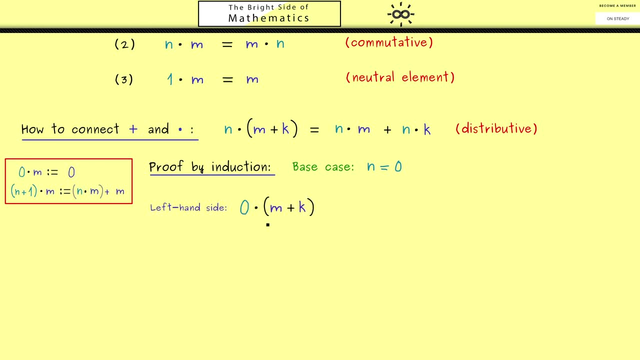 to 0.. Of course, for the induction proof we will need the recursive definition of the multiplication. Therefore, you find it here in the red box again. Now for the base case. let's calculate the left hand side and the right hand side, where we put. 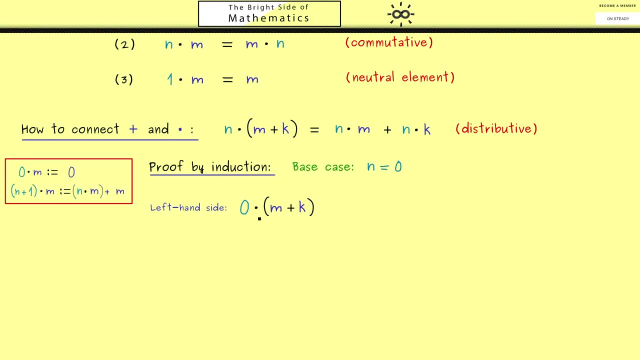 in 0 for n. Here, 0 times any natural number is simply defined as 0.. Similarly, on the right hand side we have 0 plus 0. And, of course, by the definition of the addition, this is also 0.. Now, since left hand side is equal to, 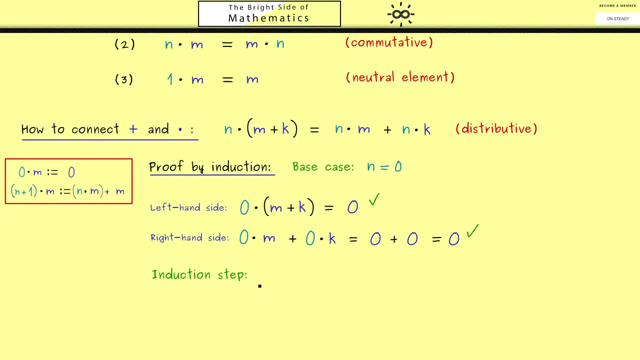 the right hand side. the base case is finished. Then let's do the induction step, which means we assume that this one is true for n and then we show it's also true for n plus 1.. The assumption that the property holds for a fixed n is often. 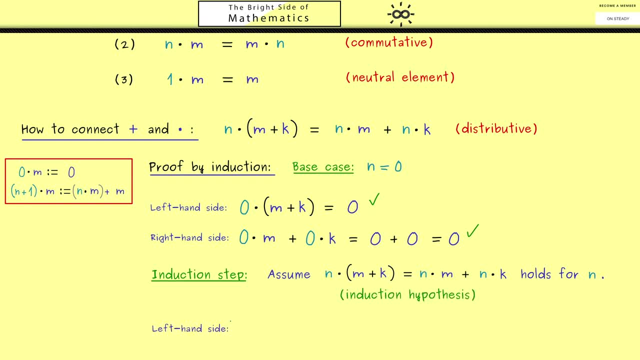 called the induction hypothesis. Ok, Then let's do the induction step by writing down the left hand side for n plus 1.. At this point you should see that in the first step, of course, the recursive definition can help us. So maybe let's mark the usage of the box. 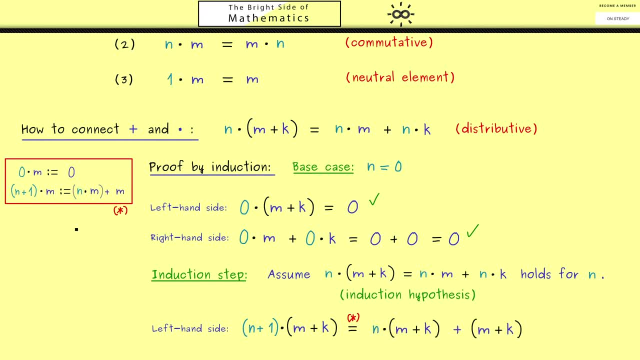 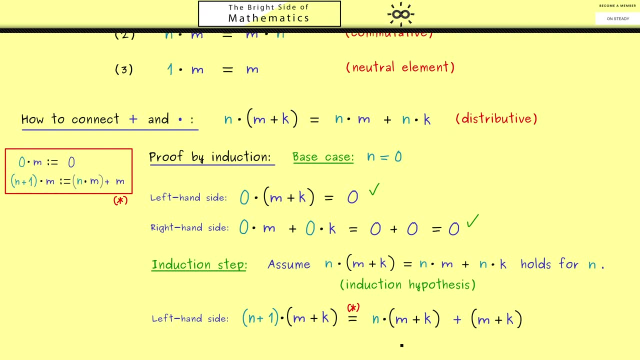 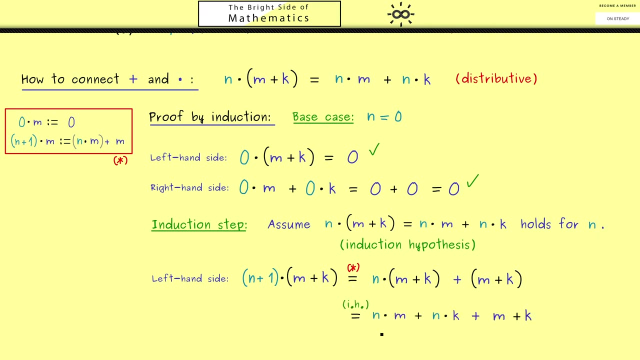 with a star. The only difference to the box we have is that the role of m here is given by m plus k. However, now in the first part of the term, you should recognize the induction hypothesis, So we can substitute this expression with this expression. Now, you should see, we just add up four natural numbers And of